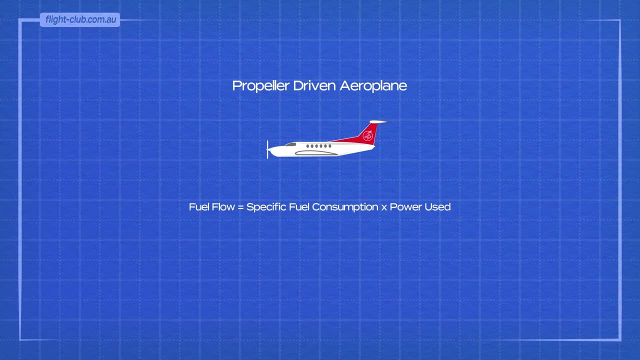 multiplied by power used For a piston engine aeroplane, this occurs at lower altitude, where the power required matches full throttle height, and for a turboprop aeroplane at medium altitude, where the true airspeed is higher and the propeller is still relatively efficient. 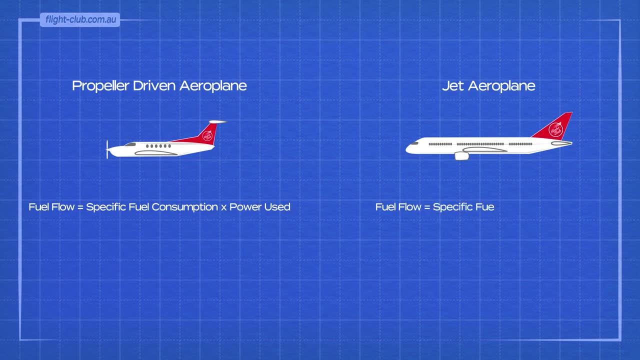 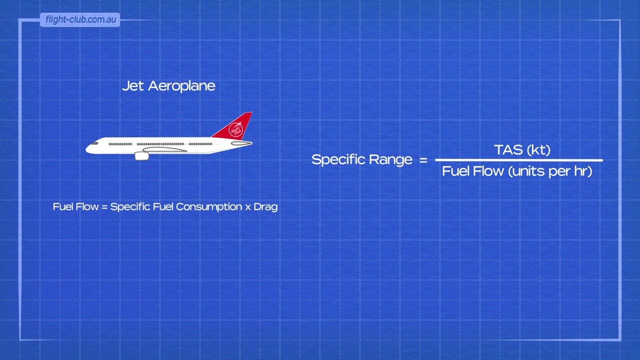 For a jet fuel flow is equal to specific fuel consumption multiplied by drag. The higher the true airspeed and the lower the power required, the greater the specific range. To maximise the range of a jet aeroplane, true airspeed must be high but at the same time, 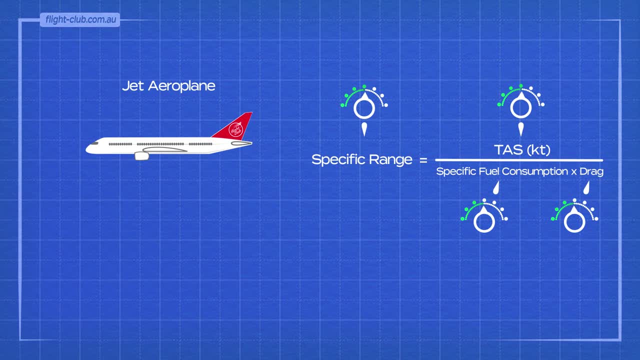 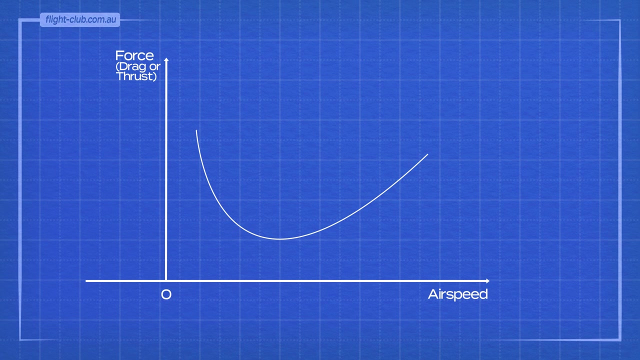 specific fuel consumption and drag must be low. This is the drag curve of a typical jet aeroplane. Drag is lowest at the bottom of the curve. This is called minimum drag speed. The drag curve is the minimum drag speed of a jet aeroplane. 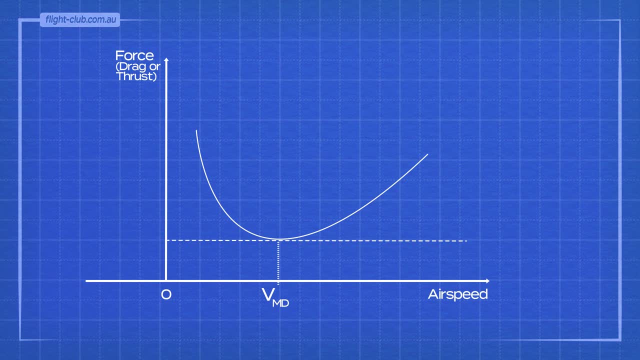 The maximum is 2.5, which is the airspeed for best endurance, For best range. however, we want the highest possible airspeed for the lowest possible drag. We want the highest drag to airspeed ratio. The maximum ratio can be found by drawing the tangent from the origin of the graph to the curve. 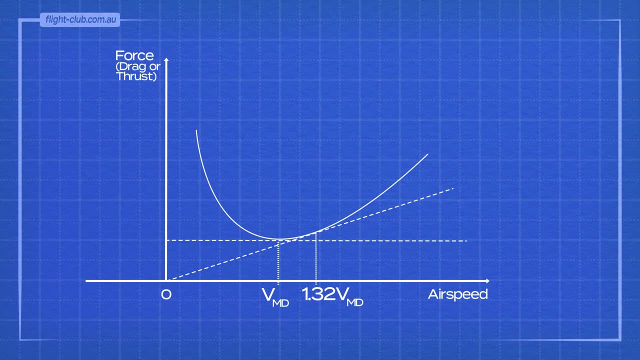 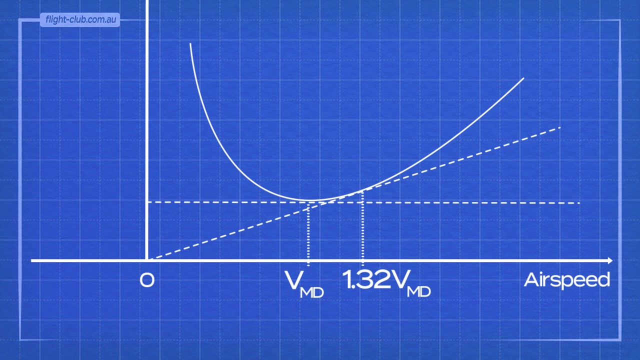 any other airspeed along the curve reduces the ratio and reduces the range. let's have a look at this concept in another way. the drag curve is relatively flat at the bottom from minimum drag speed. the airspeed may be increased significantly with only a small drag penalty. 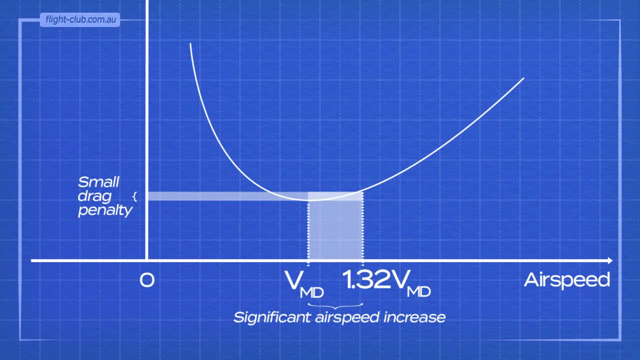 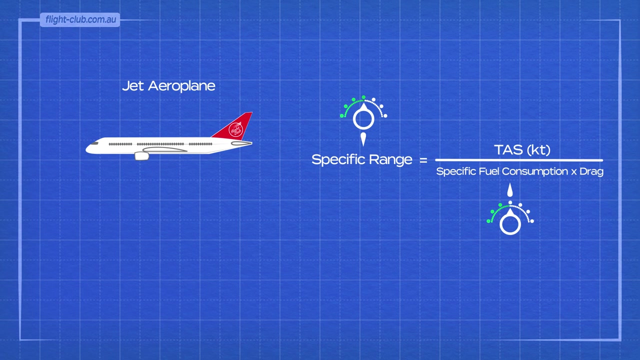 while drag increases a little, the airspeed increases significantly and this is good for maximum range. consequently, the overall effect is that there is an increase in specific range. maximum range occurs at 1.3 to minimum drag speed. there is one element remaining in the formula which we can improve on for better range: to increase range even more specific fuel consumption.